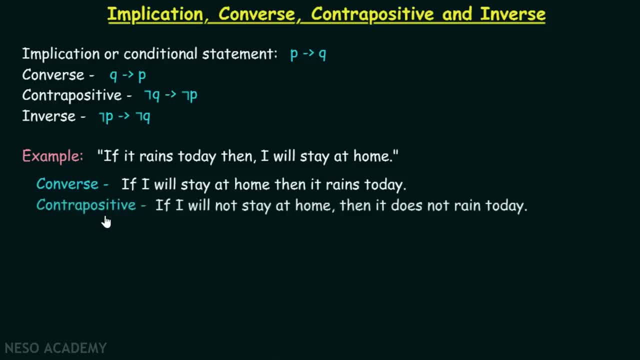 If I will stay at home, then it rains today. Contrapositive is: if I will not stay at home, then it does not rain today. Now how inverse looks like: If it does not rain today, then I will not stay at home. 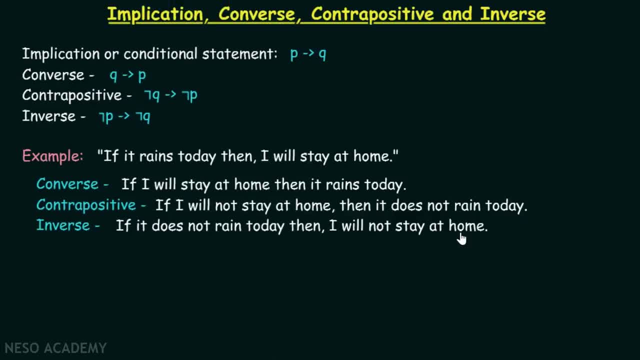 Simple. Now let's consider some facts related to implication, converse, contrapositive and inverse. Implication and contrapositive: both are equivalent. Converse and inverse: both are equivalent. Neither converse nor inverse is equivalent to implication. Now, these facts are quite important for us to understand. 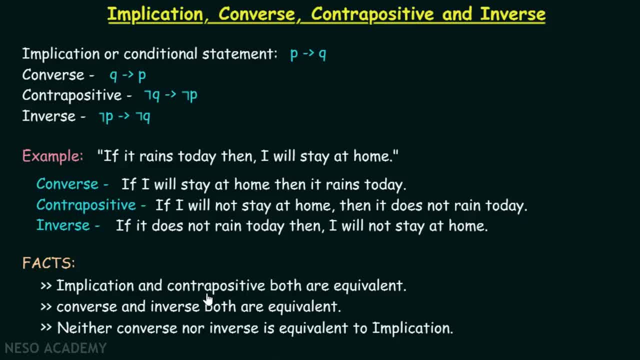 Why implication and contrapositive are equal. As we know, according to this statement, P implies Q means if P is true, then Q has to be true, Right. Or we can also say that when Q is false, then P has to be false. 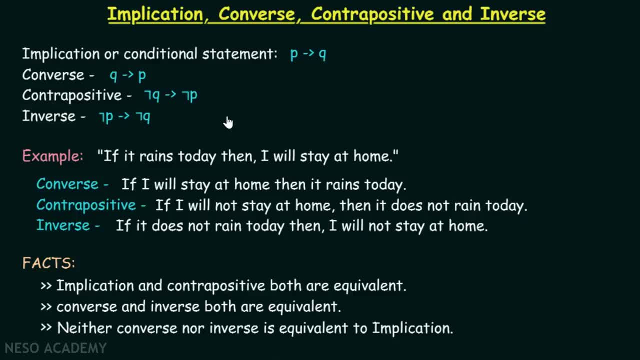 Now contrapositive just says the same in some other way. Not Q implies not P, which simply means that when Q is false, then P has to be false. Or we can also say that when P is true, then Q has to be true. 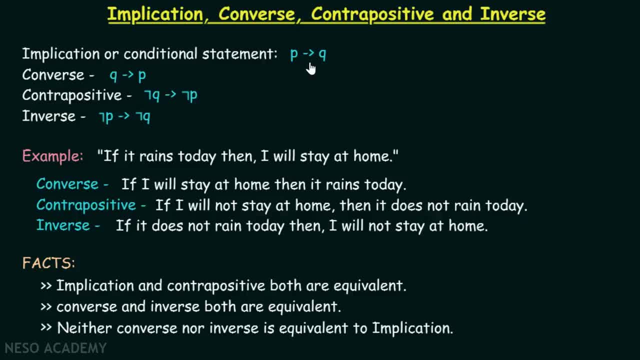 So both are equivalent, Isn't that so? Now it is not very difficult to understand that converse and inverse, both are equivalent, by using the same idea that we adopted for implication and contrapositive. And we also know that P implies Q can never be equal to Q implies P. 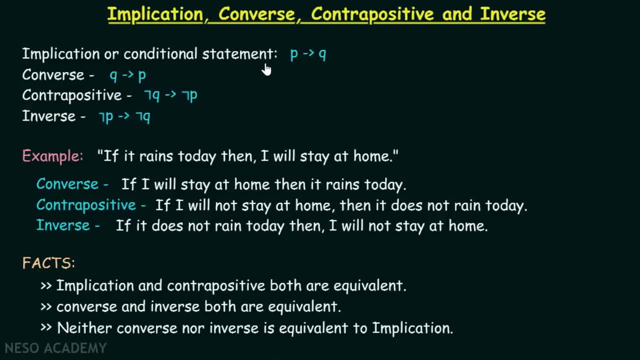 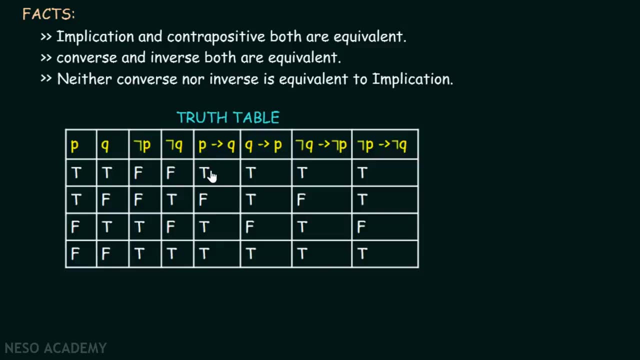 Therefore, it is not possible that converse is equivalent to implication, And similarly, we can say that inverse is not equivalent to implication. Okay, Now let's verify all these facts with the help of truth table. Now, here is the truth table for implication. 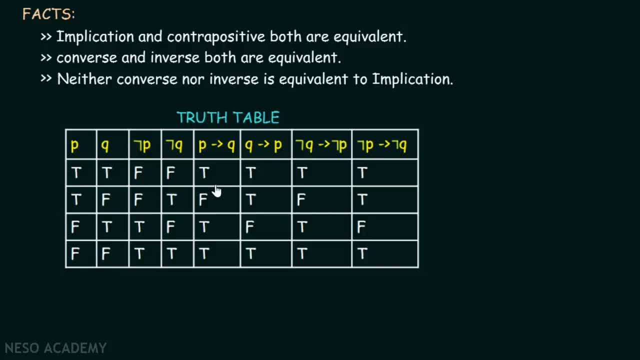 converse, contrapositive and inverse, As we can clearly see from this truth table that P implies Q is equivalent to not. Q implies not P. Right Here, the truth values are clearly the same: True, false, true, true, True, false, true, true. 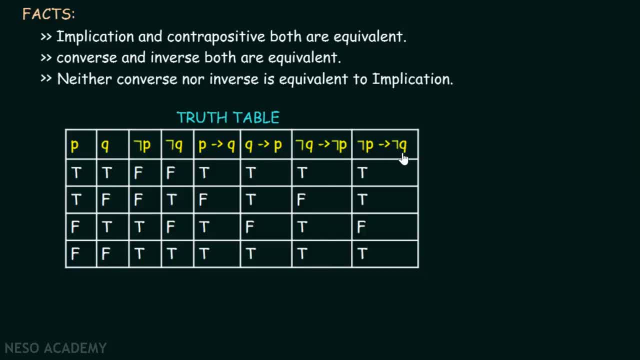 While, on the other hand, Q implies P is equivalent to not, P implies not Q. True true, false, true, True, true, false true. And neither converse nor inverse is equivalent to implication or contrapositive. This is also clear from this truth table.